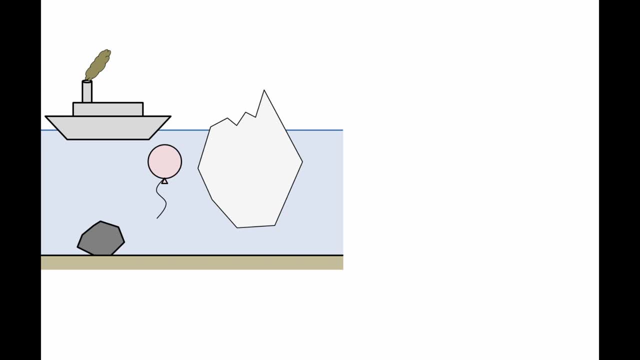 it would be easier to lift than if the rock were on dry land. Some force must be present, that is, keeping the ship and iceberg afloat, lifting the air-filled balloon to the surface and making it easier to lift the rock. If we drain the lake, the rock ship and iceberg 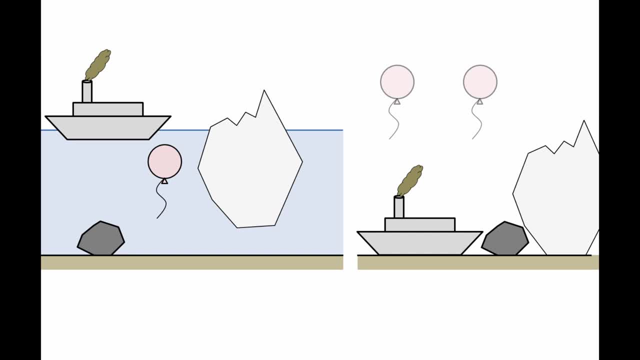 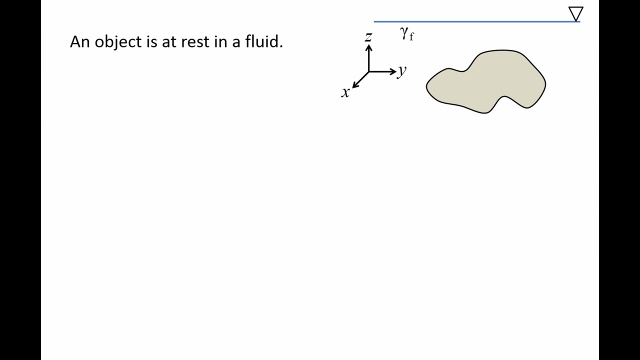 would sit at the bottom of the lake. The balloon may rise or sink depending on the gas contained inside. We want to determine the force that is causing objects to rise and float. We start by examining an object of arbitrary shape that is at rest in a fluid with specific 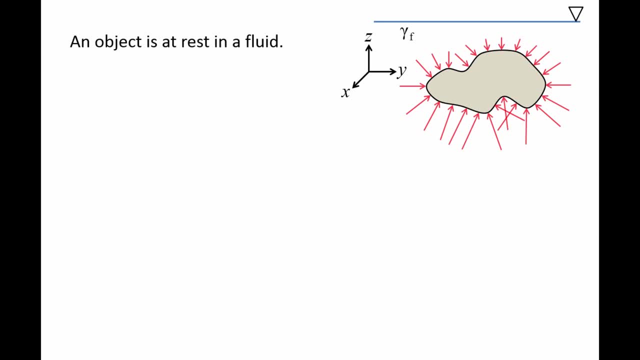 weight. gamma-f. The fluid pressure exerts a force on the entire surface of the object. This force acts normally on the surface of the object, but is not on the surface of the object. Instead, it is normal to the surface and increases with depth. 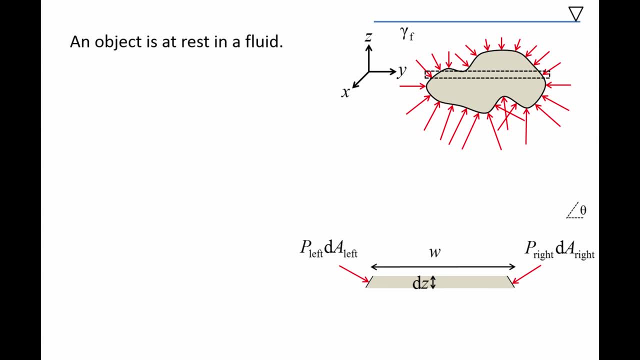 Let us examine the pressure force acting on a very thin horizontal sliver of the object. The sliver has a width W and height dZ. The force on the left side of the sliver is equal to the pressure on the left side, p, left times the small area on the left side, dA. 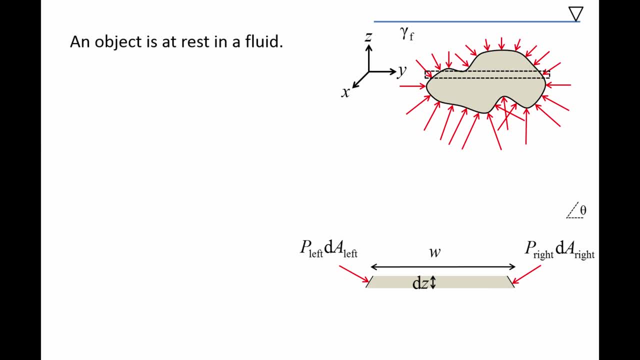 left. The force on the right side of the sliver is equal to the pressure on the right side. p. right times the small area on the left side- dA. left times the small area on the right side- dA- right. 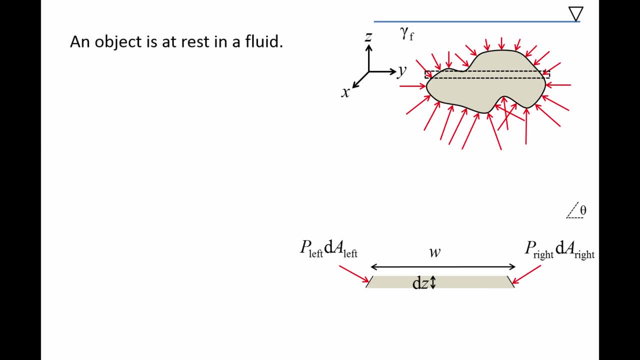 The force vectors act normal to the surface and are oriented at an angle- theta- relative to the horizontal. In general, the orientation angles may be different for each side, which means the area on the left side may be different from the area on the right side. 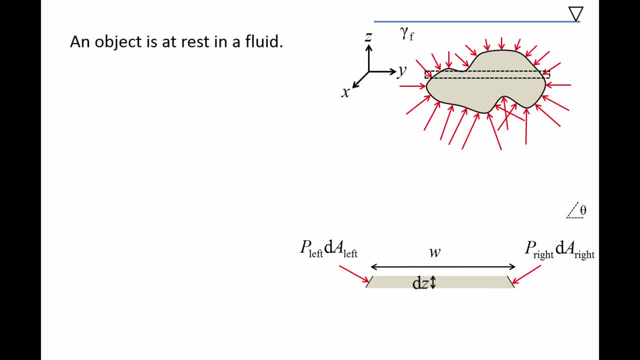 We will call the orientation angle on the left theta left and the orientation angle on the right we will call theta right. Multiplying the pressure force by cosine theta gives the component of the force in the y direction. In order to find the resultant pressure force in the y direction, we add up the net pressure. 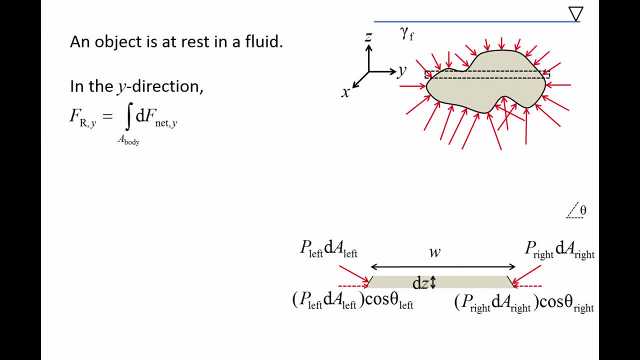 force in the y direction acting on each sliver by integrating over the entire body's surface. The net pressure force in the y direction acting on each sliver is the pressure force on the left side minus the pressure force on the right. Notice that both terms contain the quantity dA times cosine theta, which is the area projected. 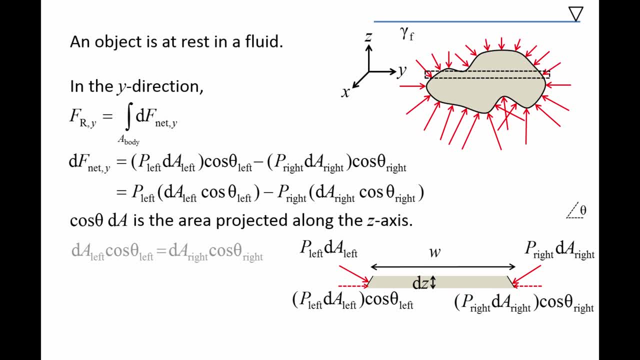 along the z axis. Since the vertical height of both sides is the same, the projected area on both sides is the same as well. That is, dA cosine theta on the left side is equal to dA cosine theta on the right side. 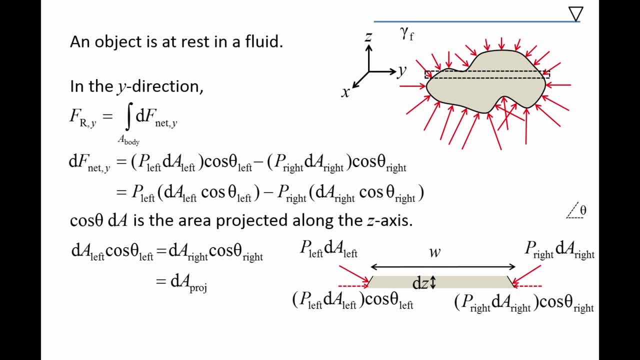 For convenience, we will call this area dA cosine theta. And that's it. Thank you for watching. Let's redraw the sliver with an equivalent picture containing the projected area. df net becomes the pressure on the left side times the projected area minus the pressure. 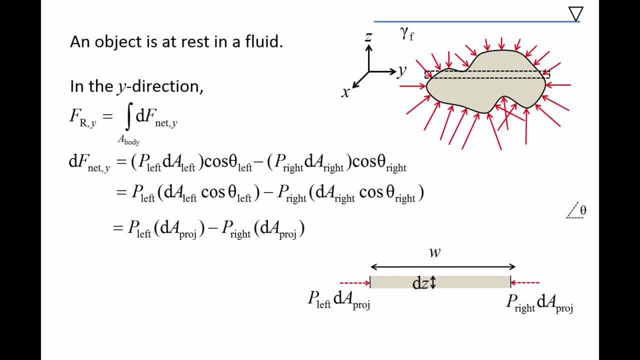 on the right side times the projected area. We can factor out dA proj, then plug in the expression for df net into the integral. The pressure on the left side is equal to the pressure on the right side because they are at the same depth. 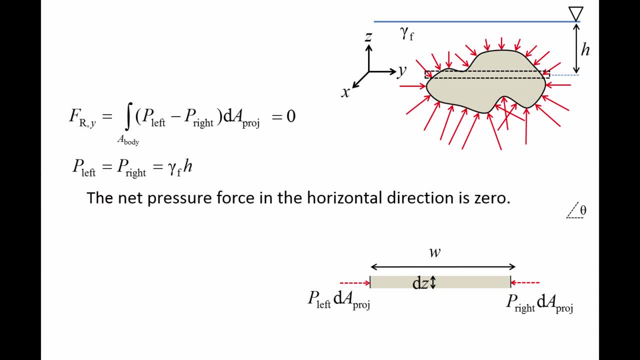 This means the net pressure force in the horizontal direction is zero. In other words, fluid pressure forces do not push an object sideways in a static fluid. Now we examine the fluid pressure force acting on a very thin vertical sliver of the object. The sliver has a width dy and a height l. 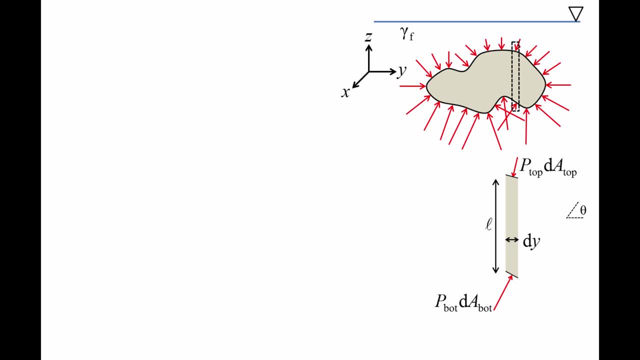 The pressure force on the top side is equal to the pressure on the right side because they are at the same depth. The pressure force on the top of the sliver is equal to the pressure on the top times the small area on the top. The pressure force on the bottom side of the sliver is equal to the pressure on the bottom. 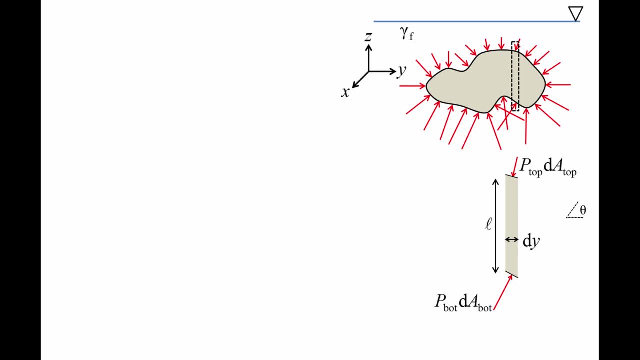 times the small area on the bottom. The force vectors act normal to the surface and are oriented at an angle theta relative to the horizontal. In general, the orientation angles may be different for each side, which means the area on the top may be different from the area on the bottom. 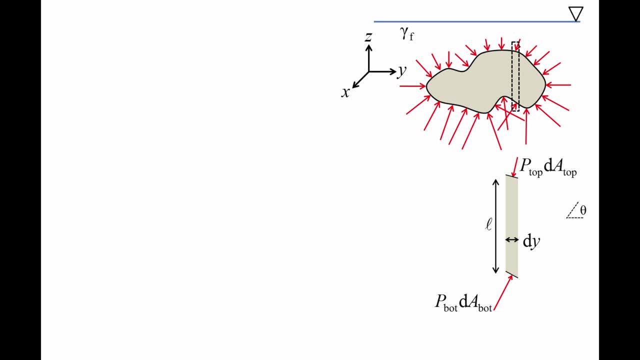 We will call the orientation angle on the top theta top and the orientation angle on the bottom will be called theta bottom. Multiplying by sine theta gives the component of the pressure force in the z direction. In order to find the resultant pressure force in the z direction, we add up the net pressure. 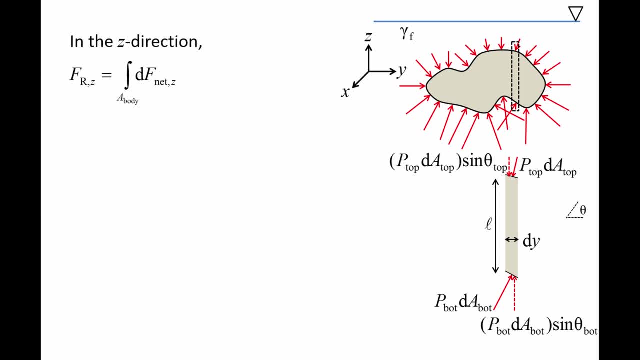 force in the z direction at each sliver by integrating over the entire surface of the entire body's surface. The net pressure force in the z-direction acting on each sliver is the pressure force from the bottom minus the pressure force from the top. Notice that both terms contain the quantity dA times sine theta, which is 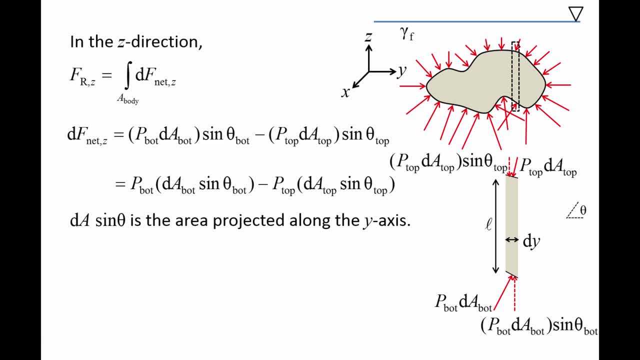 the area projected along the y-axis. Since the width of each side is the same, the projected area of both sides is the same as well. That is, dA sine theta on the top is the same as dA sine theta on the bottom. For convenience, we will call: 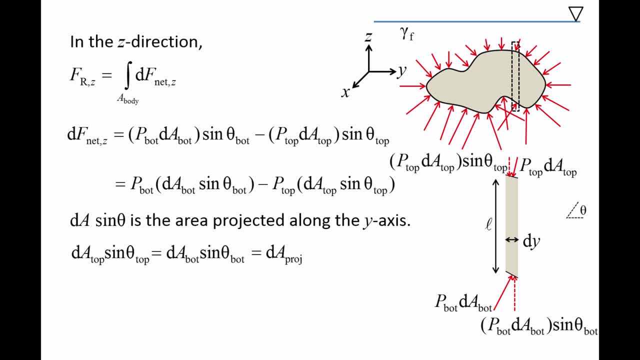 this area dA proj. Let's redraw the sliver with an equivalent picture containing the projected area dF. net becomes the pressure at the bottom times dA proj minus the pressure at the top times dA proj. We can factor out dA proj. 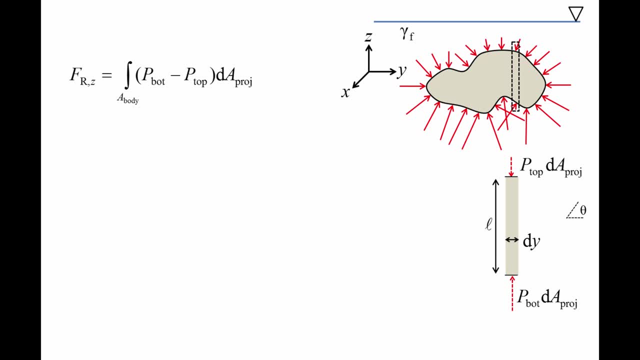 then plug in the expression for dF net- dF net- into the integral. The pressure at the top of the sliver is the specific weight of the fluid times. the depth h top. and the pressure at the bottom of the sliver is the specific weight of the fluid times, the depth h bot. Plug in the. 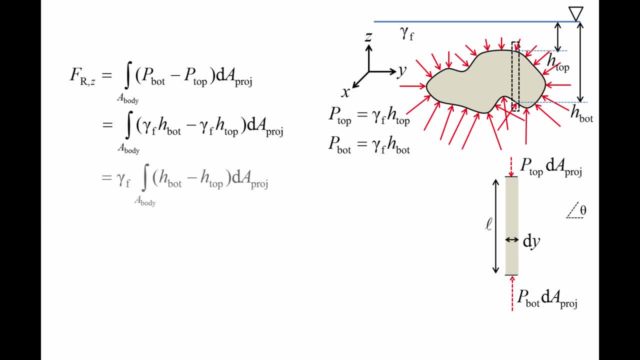 expression for the pressures and pull out the specific weight of the fluid from the integral, because it is constant. The difference in depth between the top and bottom of the sliver is the length, L. L times dA. proj is the volume of the small sliver, dV. 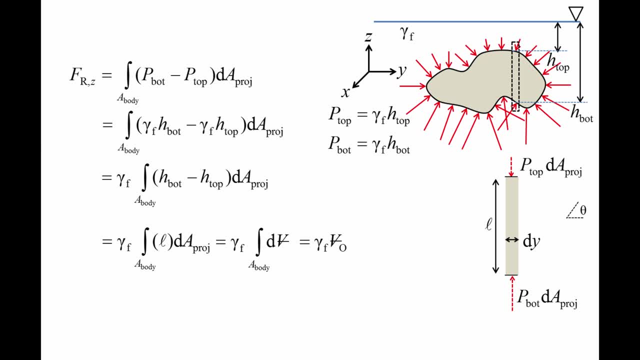 Integrating dV over the entire body gives the volume of the object which we will call Vo. We now have an expression for the resultant force. This force, which is caused by the fluid pressure gradient, is called the buoyant force and is denoted as Fb. The buoyant force points upward. 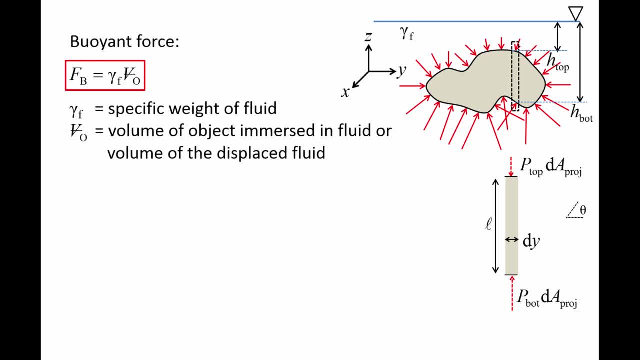 The magnitude of this force is the specific weight of the fluid. gamma F times the volume of the object immersed in the fluid. Vo. Vo also could be thought of as the volume of fluid that is displaced by the object's presence. That means the buoyant force is.